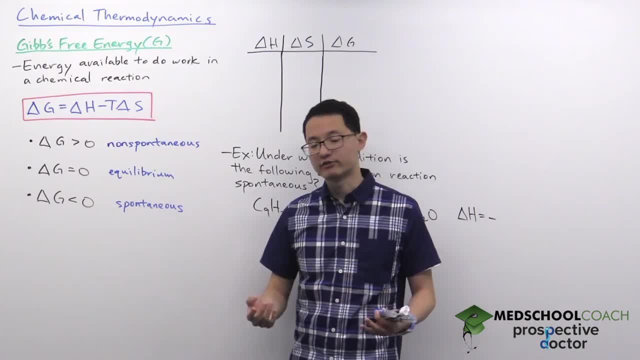 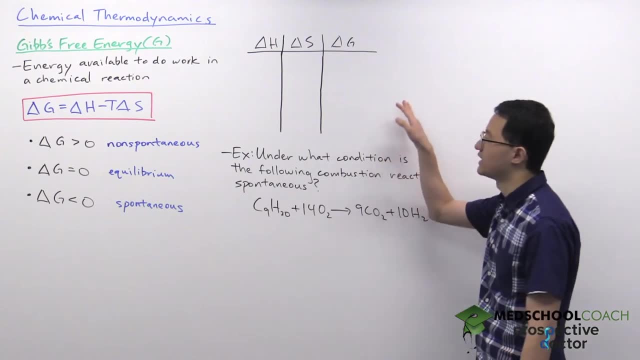 where a reaction will be non-spontaneous And there are other reactions that are always spontaneous and others that are always non-spontaneous. We can see how this works with this table right here, where we'll look at different combinations of enthalpy change and entropy change. 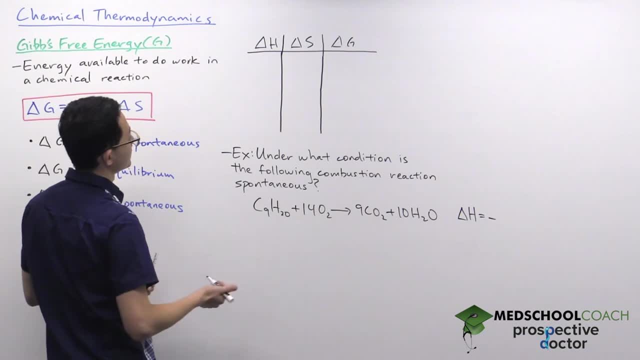 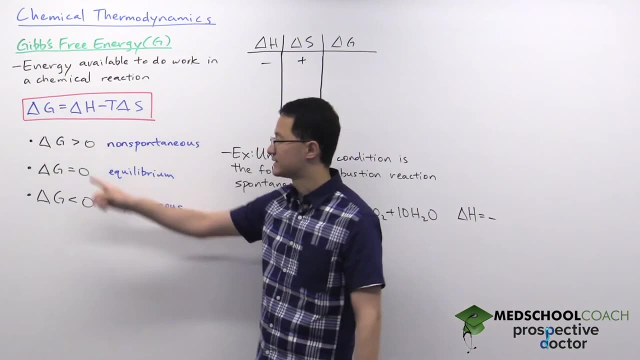 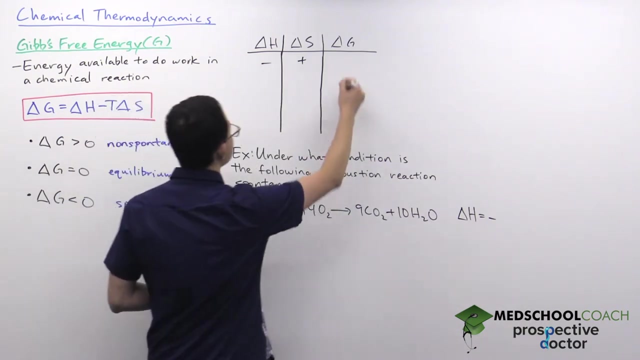 So, for instance, let's say we start off with reactions whose enthalpy change is negative And entropy change is positive. In this case, since the enthalpy change is negative and you are subtracting a positive value, then the Gibbs free energy change is always going to be negative. 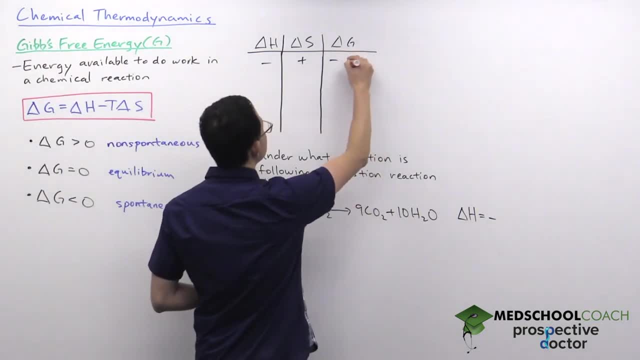 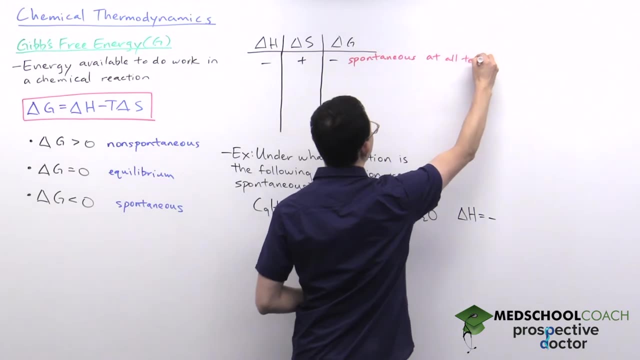 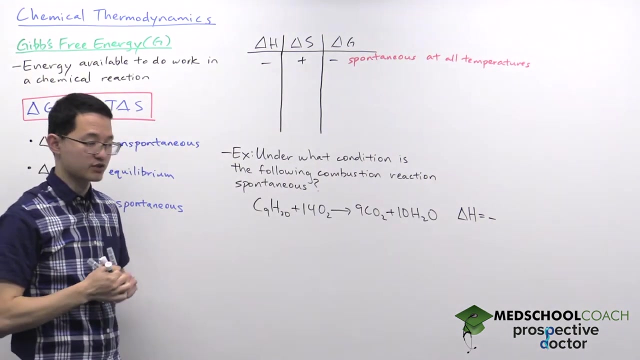 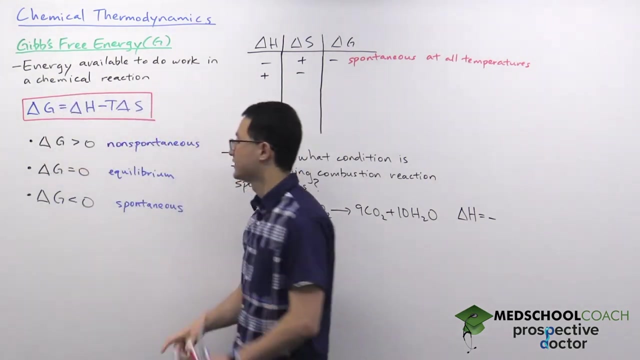 And in these situations our reaction is spontaneous at all temperatures. So now we can consider the opposite. So if we have a reaction that is endothermic and the entropy change is negative, then you have a positive value and you're subtracting a negative value. 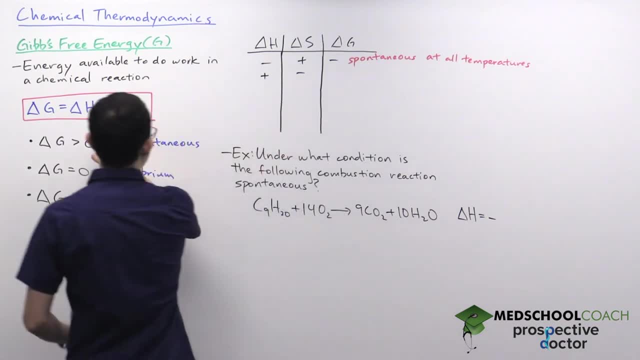 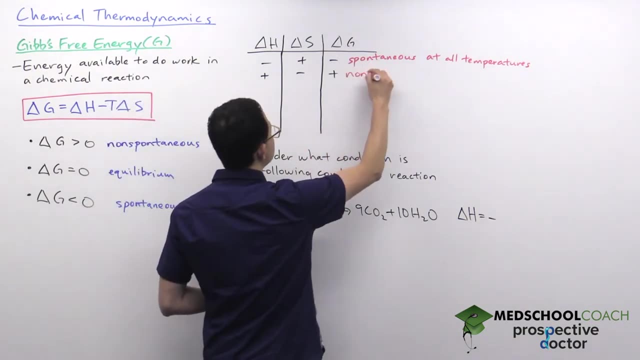 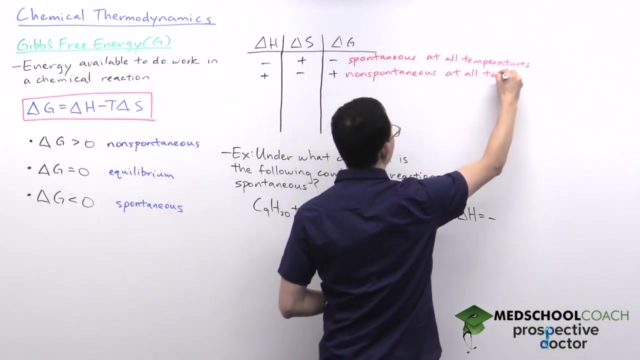 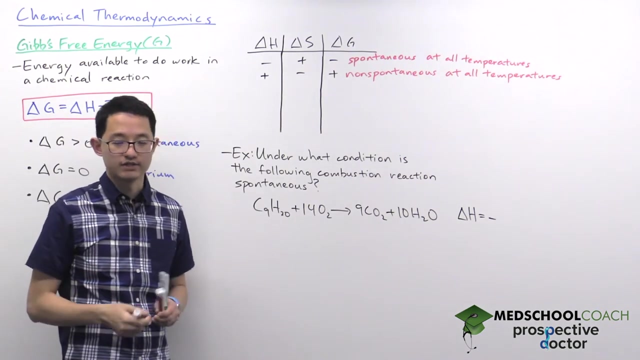 That's double negative, which is addition, So that will always give you a positive Gibbs. free energy change, meaning this reaction is non-spontaneous at all temperatures. Okay, So now we can consider more complicated situations. So let's say we have a reaction where the enthalpy change and the entropy change are. 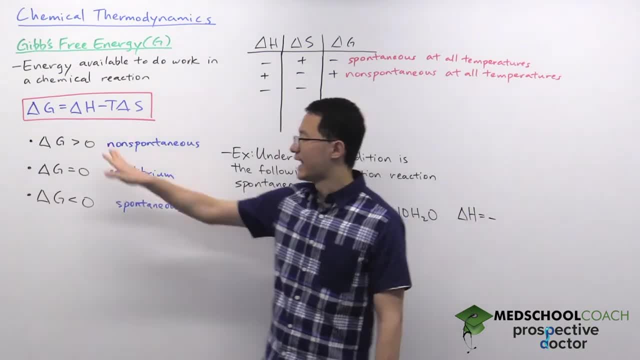 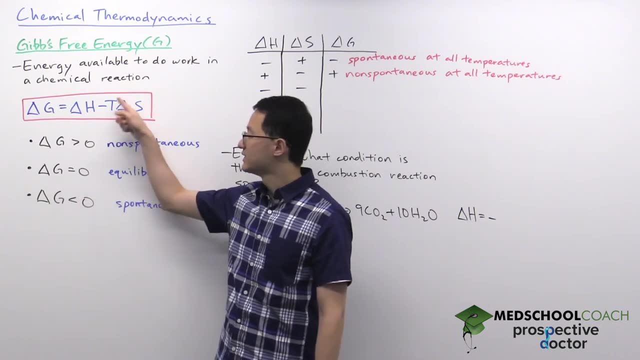 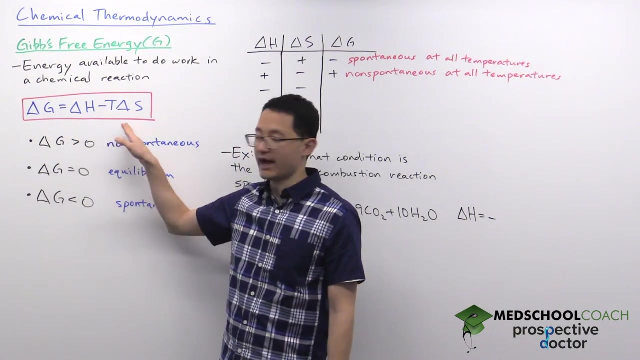 both negative, In this case the enthalpy change. this is a negative value and we are subtracting a negative value. So this temperature entropy term is positive, And this is where it gets tricky. The enthalpy term is negative. 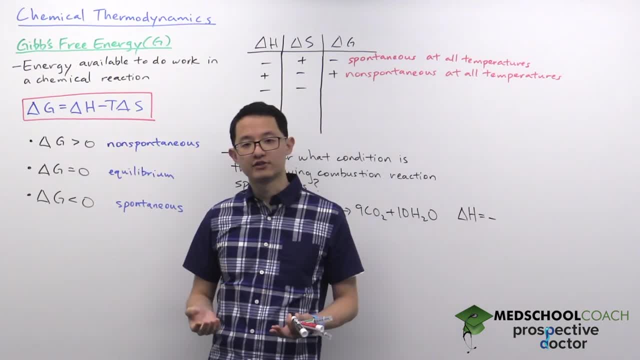 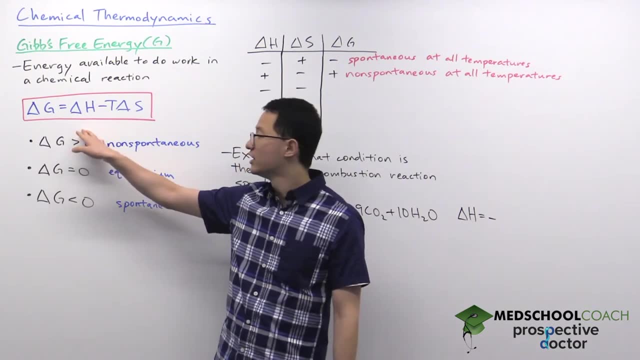 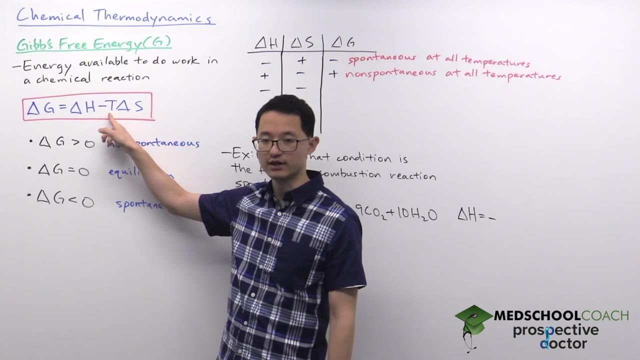 The entropy term is positive. Whether or not your reaction is spontaneous, then depends on which term is larger. Is the negative enthalpy term larger or is the positive entropy term larger? And, as it turns out, this depends on the temperature, because at low temperatures the entropy term 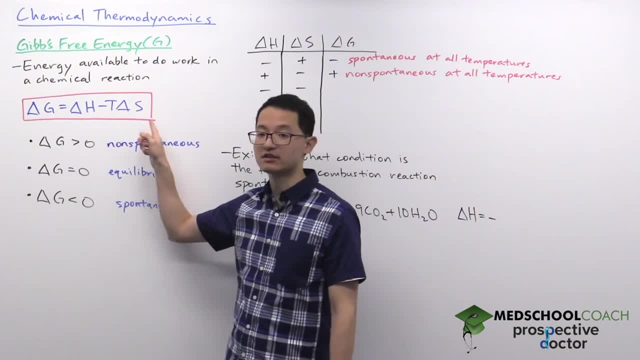 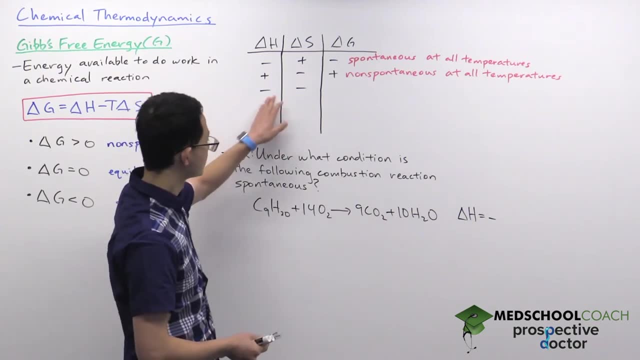 is small. At high temperatures the entropy term is large, And here the entropy term is small. And here if we want our reaction to be spontaneous, then we want low temperatures, So the enthalpy term is larger than the entropy term. 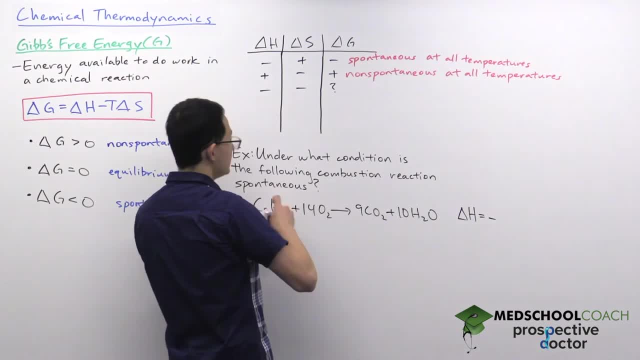 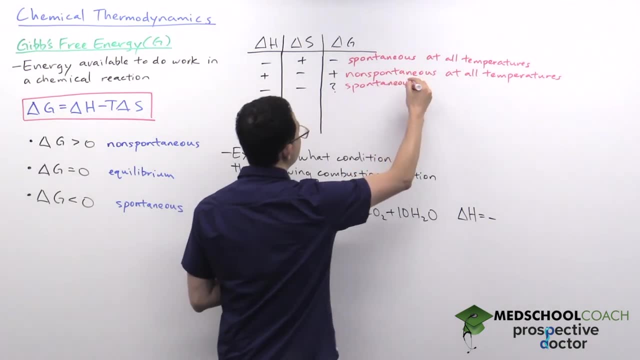 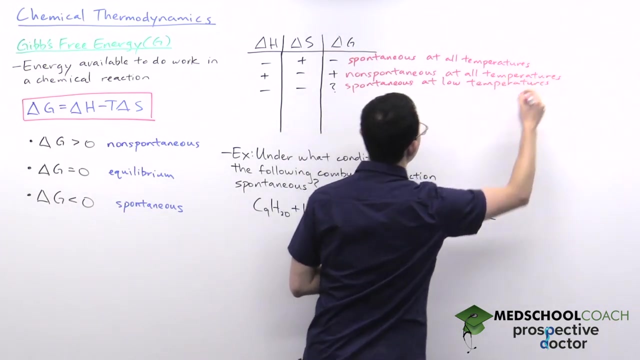 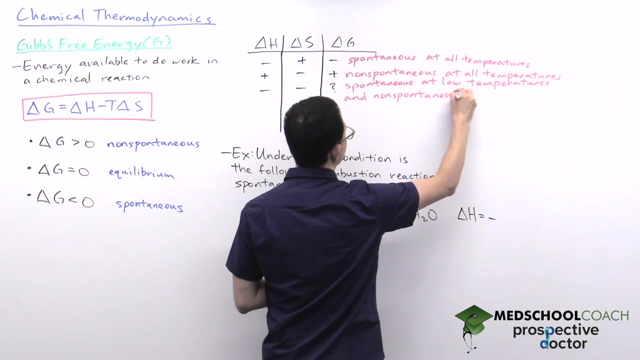 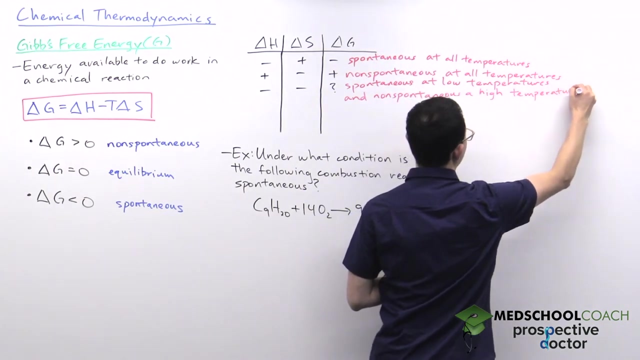 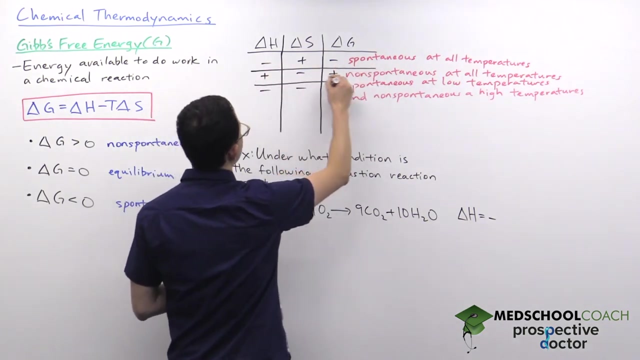 So here the Gibbs, free energy actually depends and it's going to be spontaneous at low temperatures And non-spontaneous At high temperatures. So finally, we can consider the last situation. In the last situation we have a reaction where the enthalpy change and the entropy change. 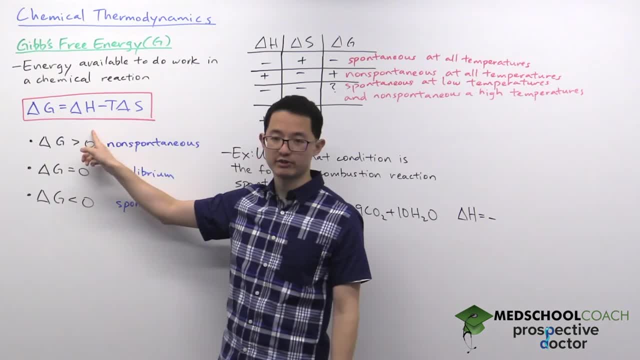 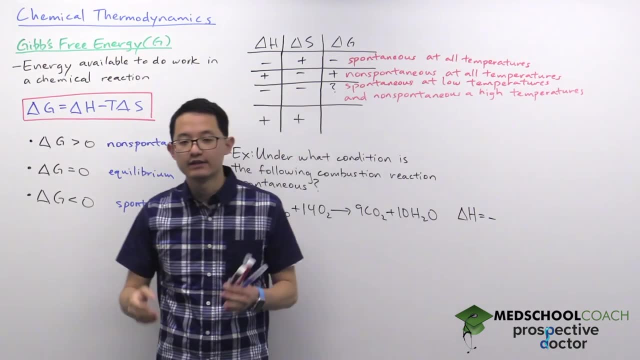 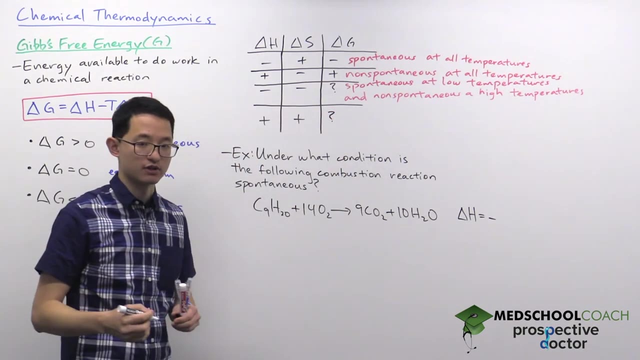 are both positive. In this case, enthalpy change is a positive term. You're subtracting a positive term, So this entropy change is a negative term. Again, you have both a positive term and a negative term. So the Gibbs free energy change is going to depend on temperature. 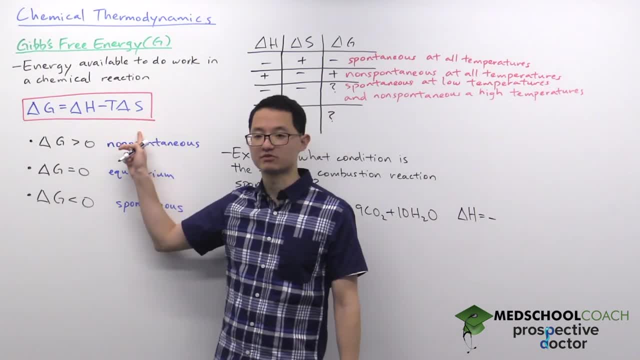 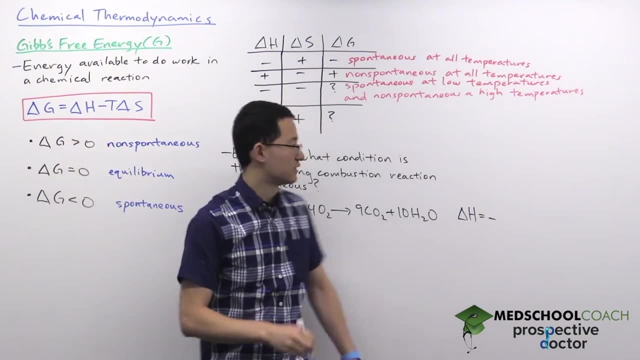 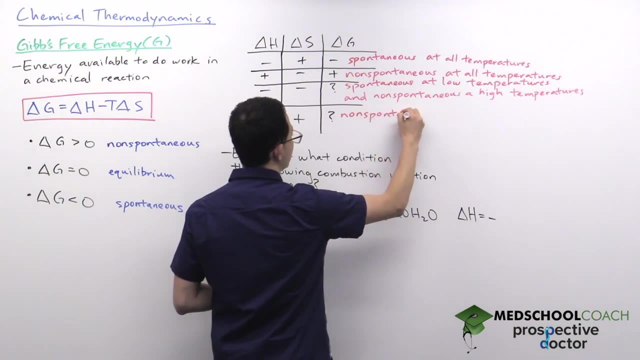 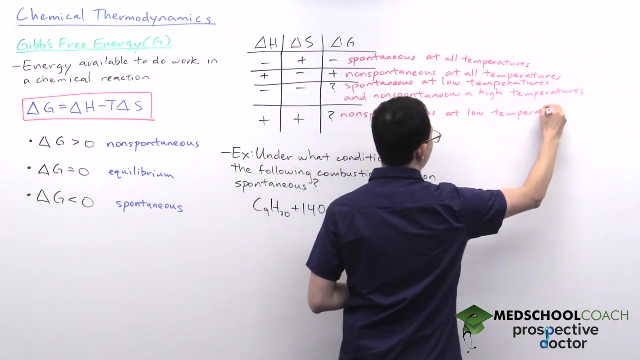 In this case at low temperatures, the negative entropy term is small, So the reaction will be endergonic because the enthalpy term is positive. So here our reaction is non-spontaneous at low temperatures And spontaneous at high temperatures. 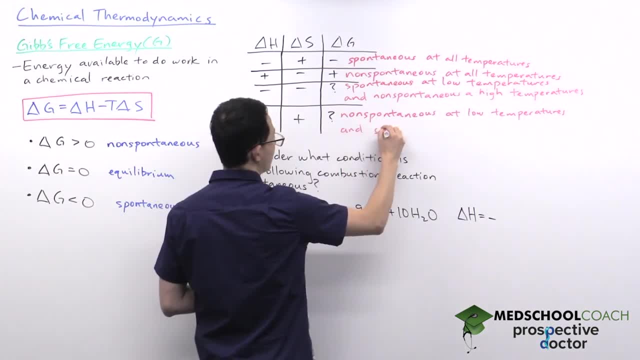 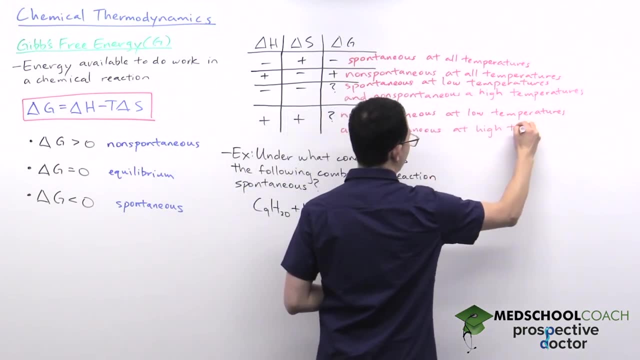 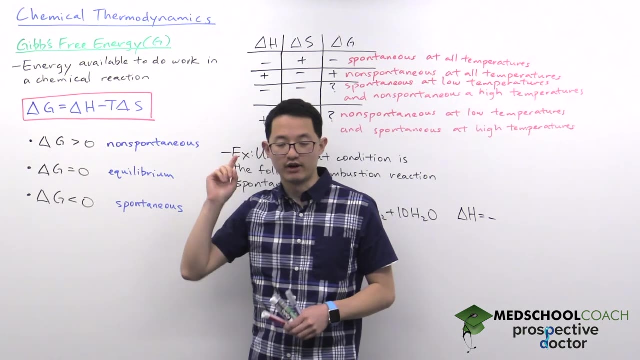 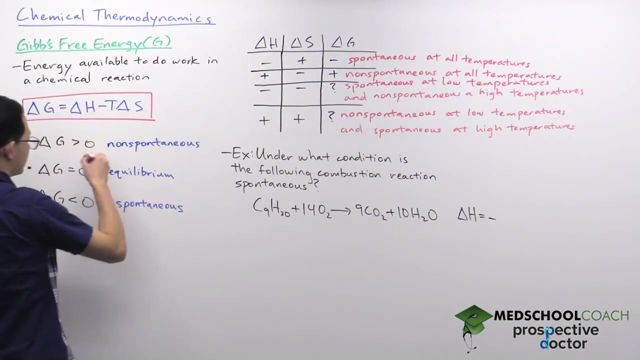 You'll also note, in this last example I introduced a new term: endergonic. Endergonic is to refer to a reaction. Endergonic Endergonic is to refer to a reaction. Endergonic is to refer to a reaction whose free energy change is positive. 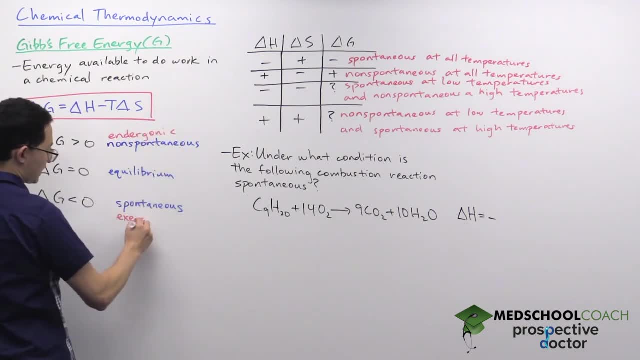 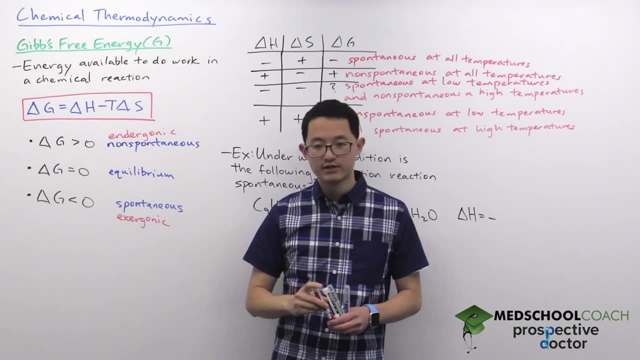 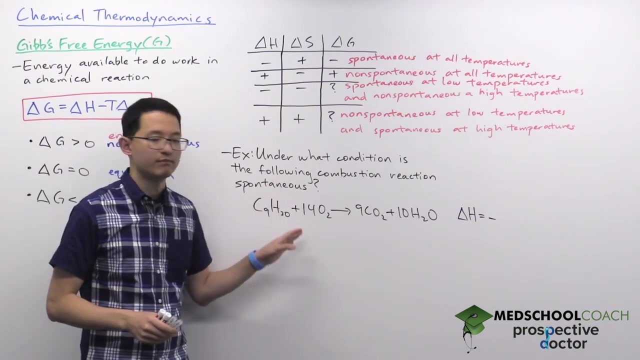 And the opposite is exergonic. So exergonic reactions are spontaneous because they have a free energy change that is negative. So now that we've gone through these different situations, let's take a look at an example. We want to know under what conditions is the following combustion reaction spontaneous?